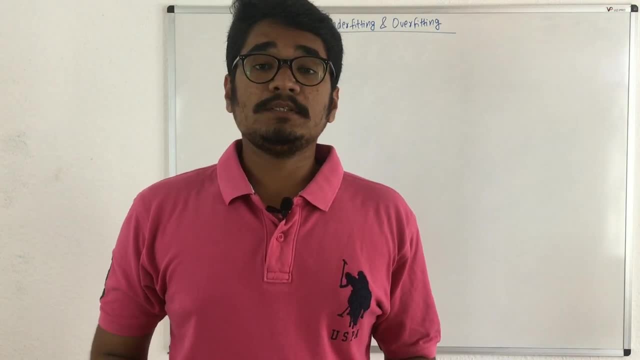 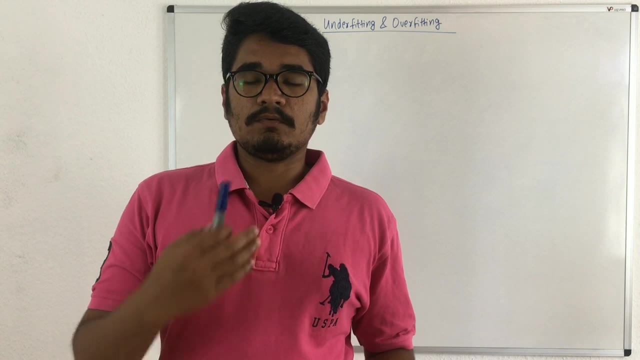 Hello people, welcome back to my channel. So today in this video we'll be seeing what is model overfitting and underfitting in decision trees. So we have already seen what are decision trees and what is decision tree capable of in doing machine learning. So today let us understand. 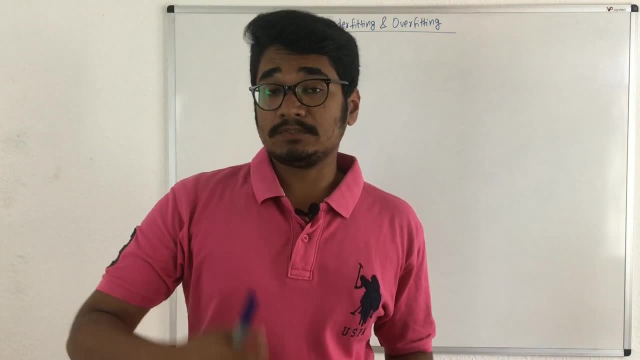 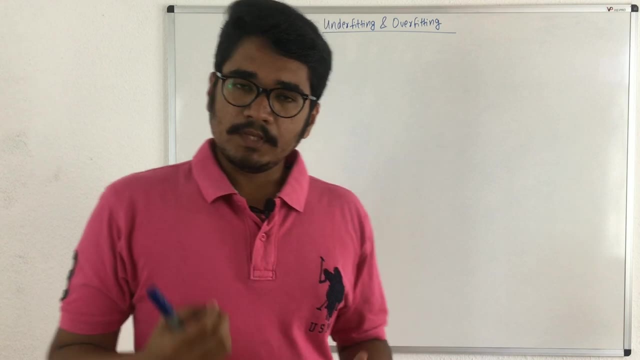 the two most important terms in machine learning or which are associated with machine learning, particularly with decision trees. that is, we have the underfitting and overfitting, So let's get started. So, basically, what is meant by fitting? first of all, so fitting. 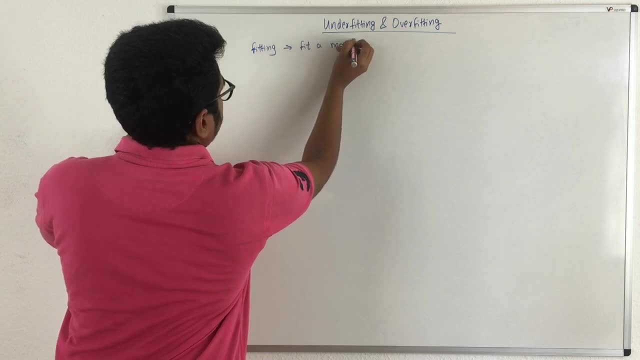 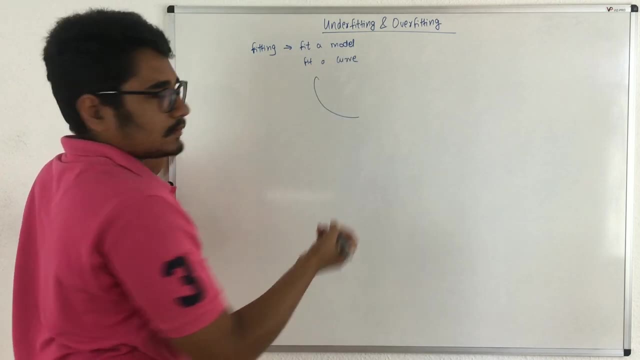 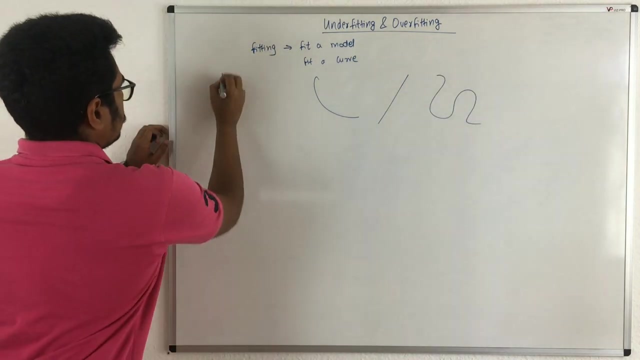 is to fit a model, Which means you mean to fit up curve. So a curve can be something like this, or it can be like this, or it can be some in a random shape, So you need to fit a curve. So this is represented in two dimensions, as y axis and x axis. 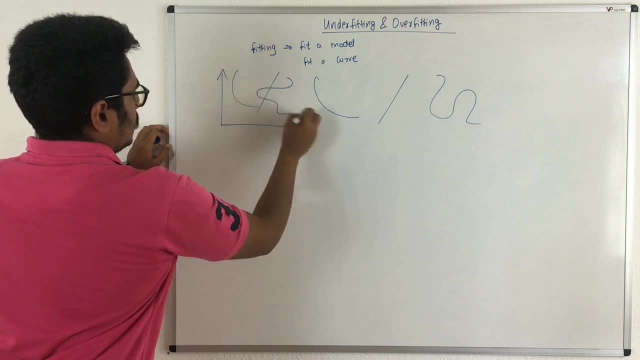 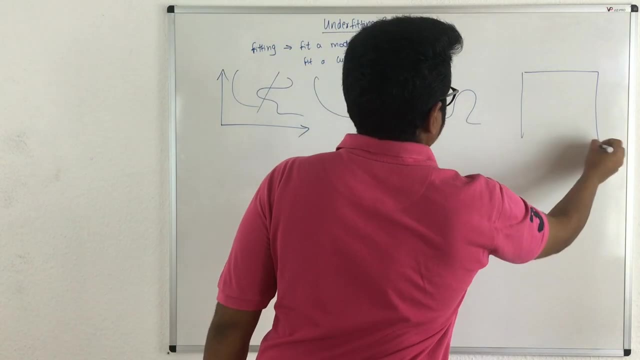 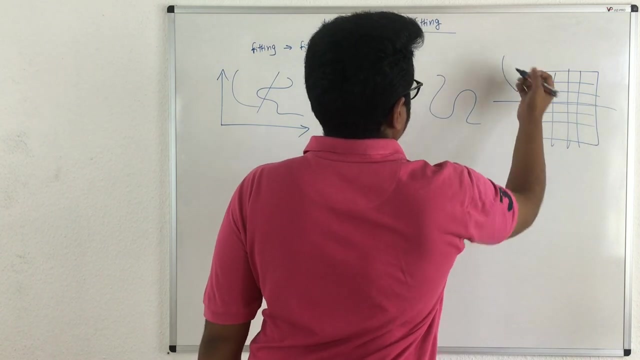 And you have to plot this curve somewhere like this, and it would be in this: Now what happens is that you have your data set, So it's divided into a number of rows and a number of columns, and you partition into some say, for example, 67%, and you have 33%. 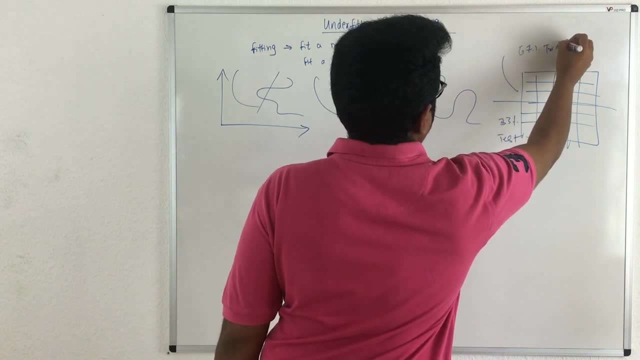 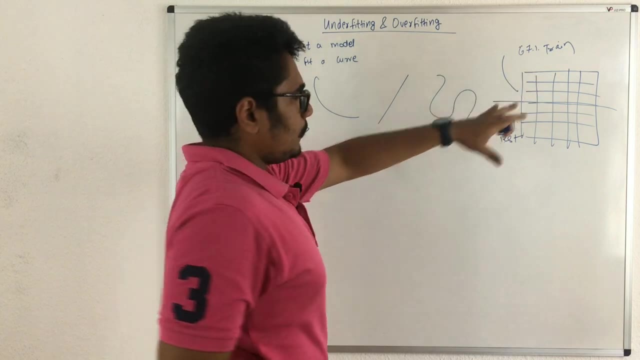 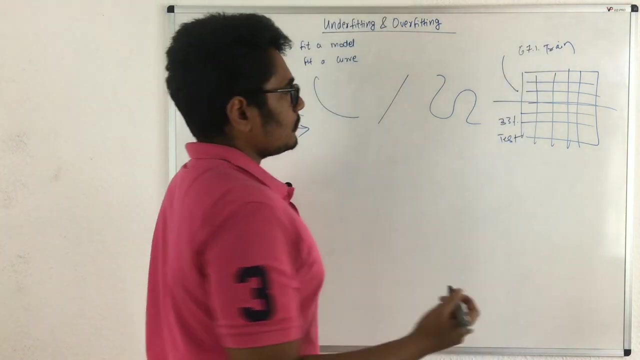 So this will be your test set, This will be your training set, and this part you train used to create your model, or you used to develop your model, and this part you just used to validate your develop model. So in this process you will get some kind of error. So 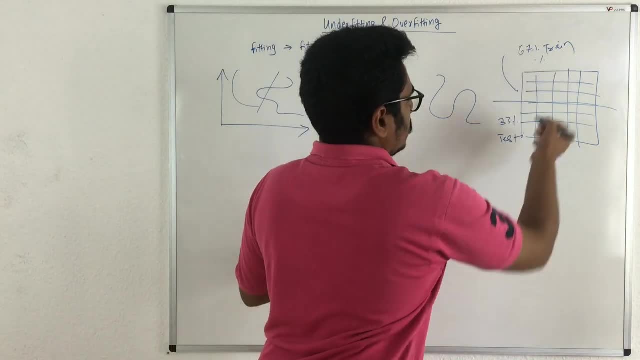 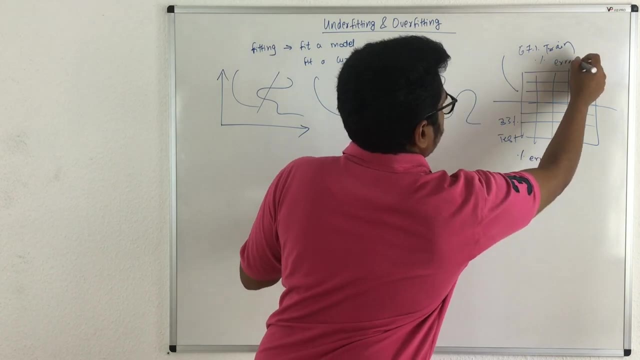 that kind of percentage error. you mark it and you obtain and you keep it aside and here also you will get some percentage error. So these are two errors which you do when you train your model. So you have some training error as well as you have some training error as well as you have some. 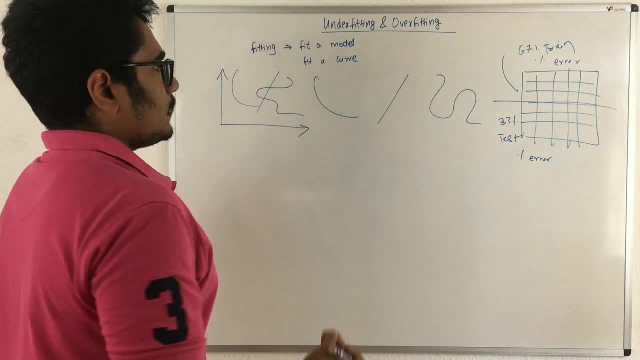 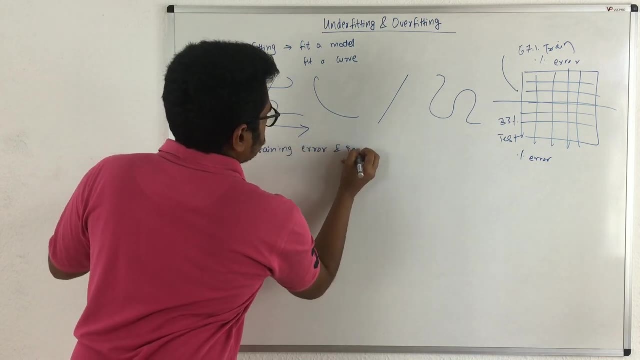 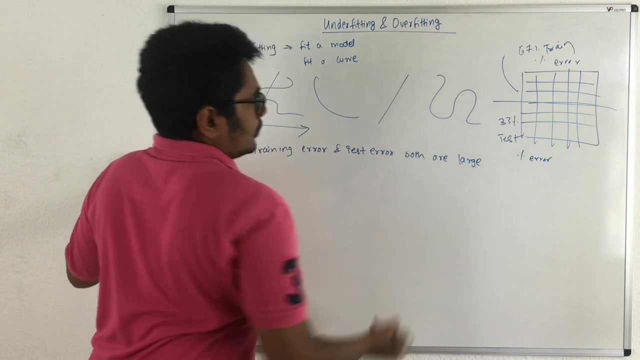 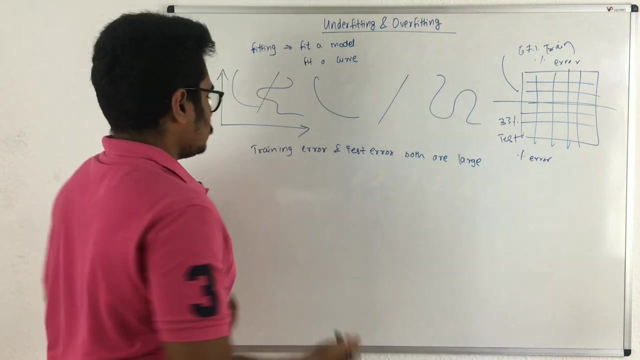 test error. Now what under fitting means is that when your training errors and test errors- both are large, means it's very high. It's not unacceptable. in that case, you call it as under fitting means. this majorly happens when your developed model developed class. 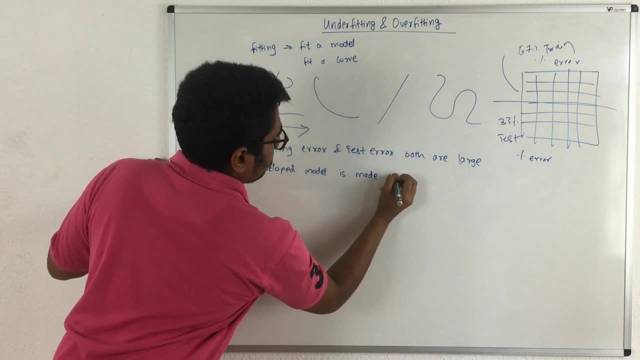 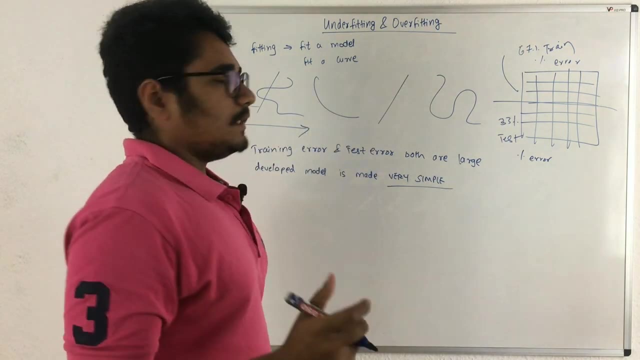 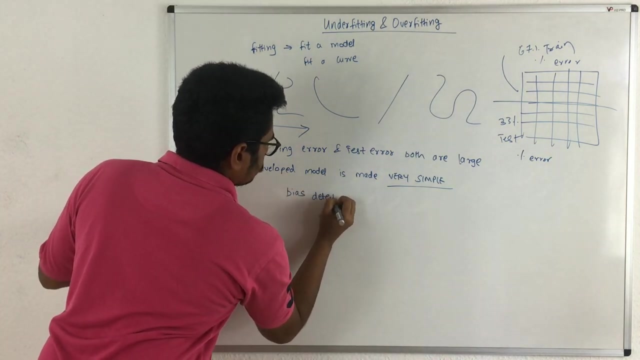 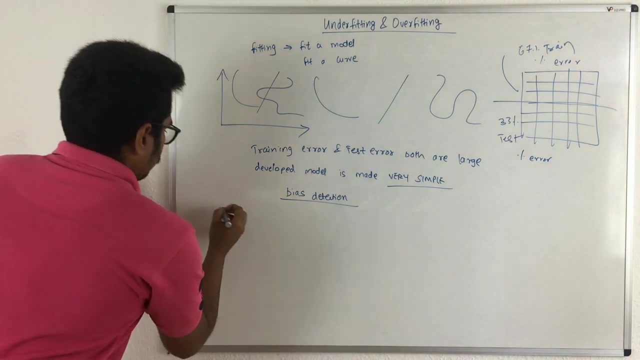 So the classification model is made very simple. So in this case under fitting happens. so under fitting is mainly detected with the help of bias detection. So various techniques are there in order to determine the under fitting. So say, for example, you have something like this: 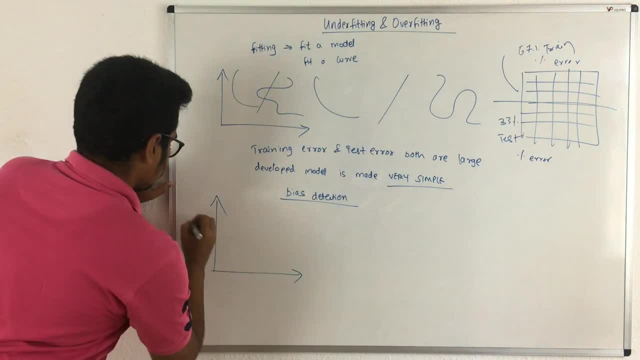 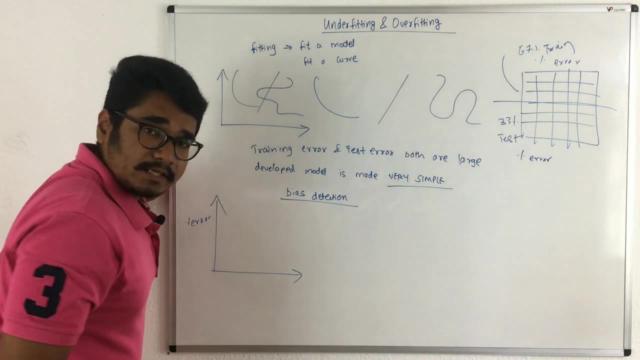 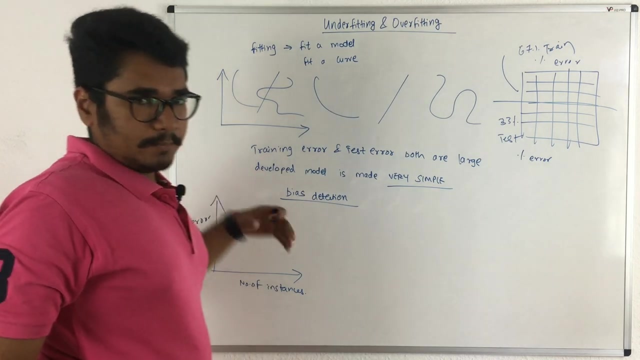 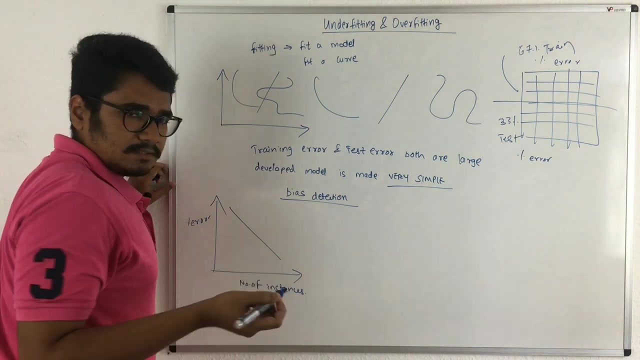 So here, what you have on the y-axis, just plot the percentage error which you have from this part, that is, training or tester, and on the x-axis what you have is basically the number of instances which is used for building your model. So under fitting curve, say, for example, it's like this, and you have some instances, say 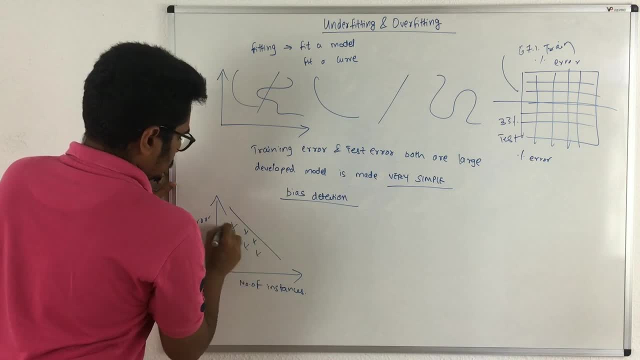 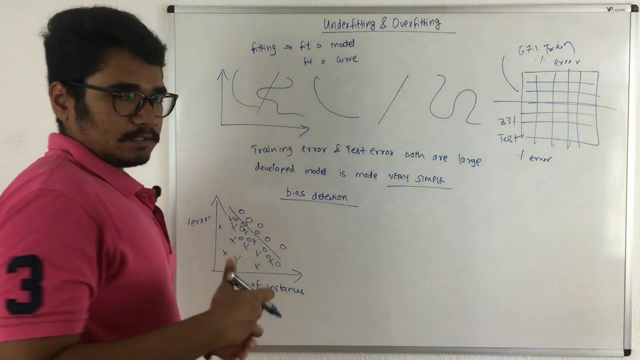 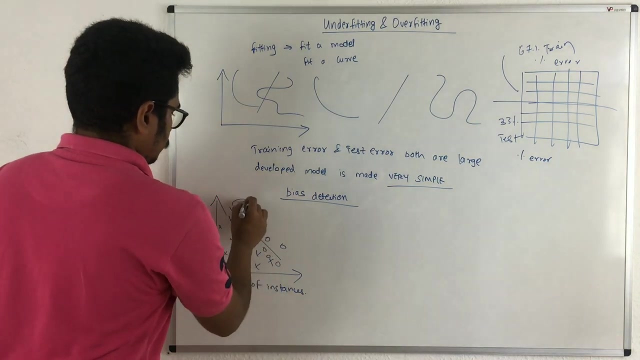 you have some labels like this and some labels like this, so some part of it may fall in this category and some part may fall above this line. So this is not well fitted, or this curve is not well fit into this particular graph. So this is mainly the description of goodness, of a fit. 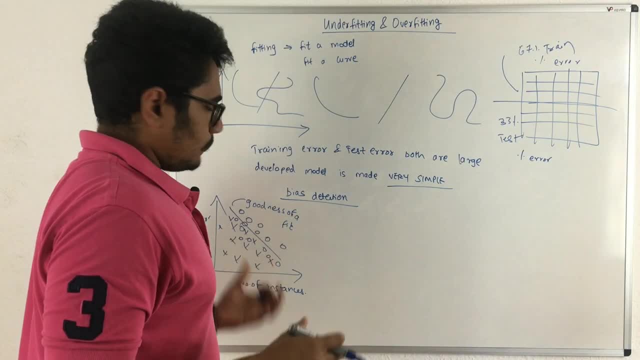 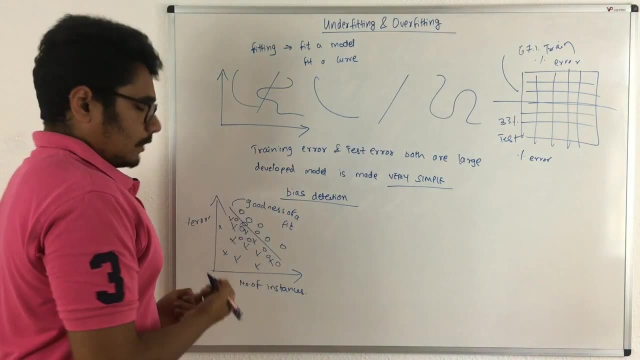 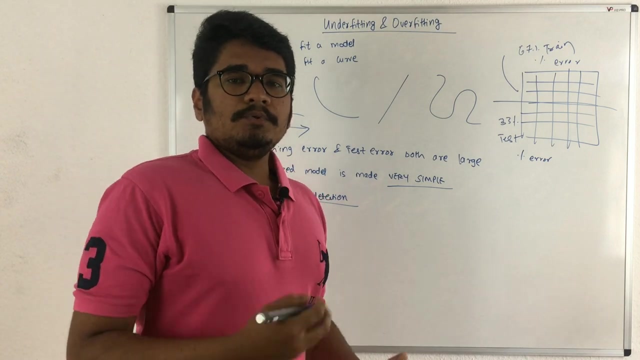 Minsk how well the given observations or given samples are being fitted into that particular curve. So this is the case of underfitting. now, what do you mean by overfitting? now you have this kind of model, so you build your model and you have your training going very well. 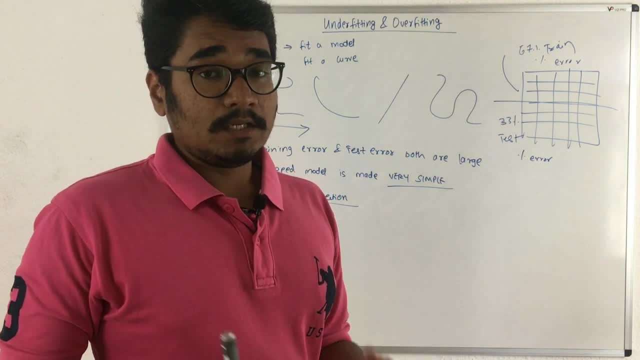 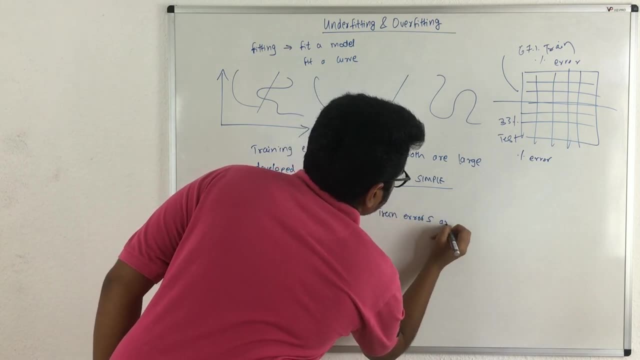 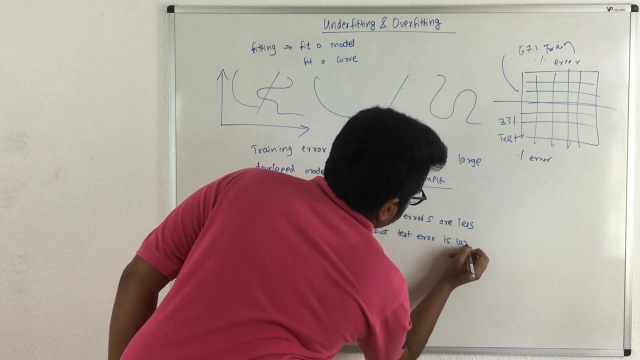 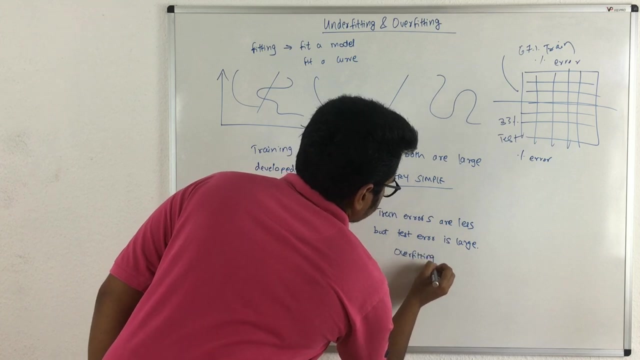 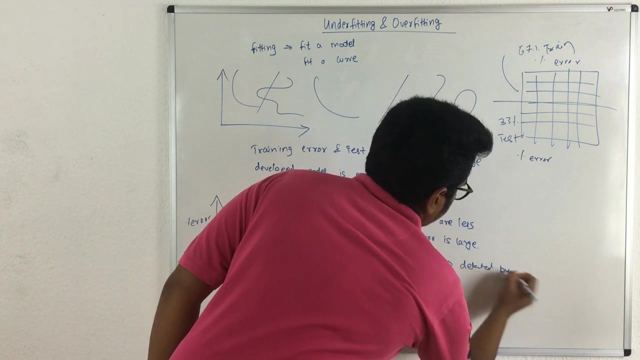 So if the training errors are very good, but the test errors are very large. So if the train errors or the training errors are less, but test error is large. So in this case what happens is you have the problem of overfitting. So overfitting is mainly detected with the help of variance. 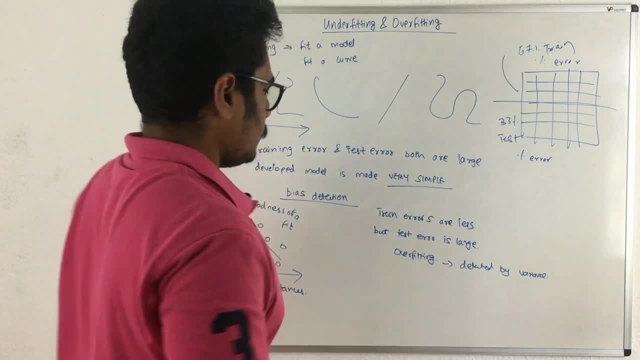 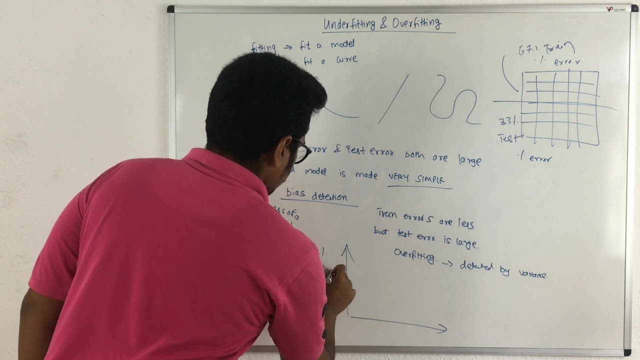 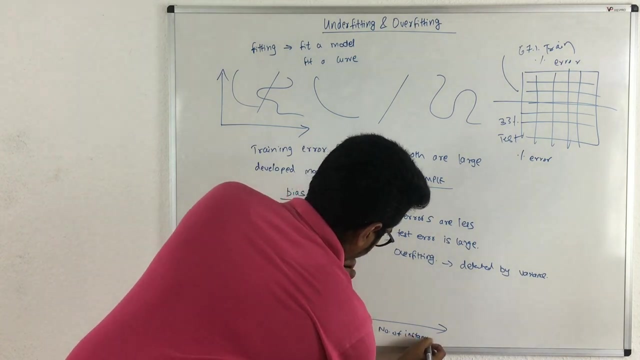 So you have This test for detecting the overfitting of a curve. So the curve. say, for example, you have the similar curve and you have percentage error on the y-axis and on the x-axis you have the number of instances. So say, for example, you have some instances like this: